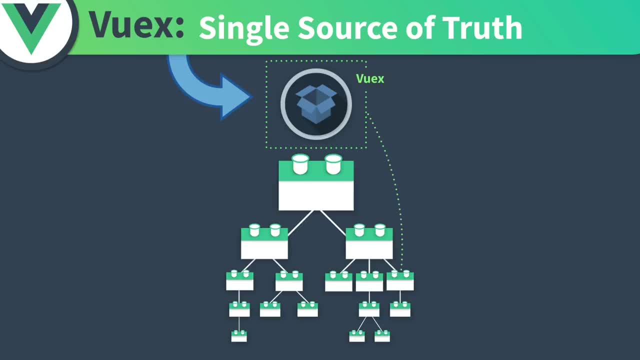 This is what Vuex provides, and every component has direct access to this global state. And just like the Vue instances data, this global state is reactive. So when one component updates the state, other components that are using that data get notified, automatically receiving the new value. But just consolidating data into one 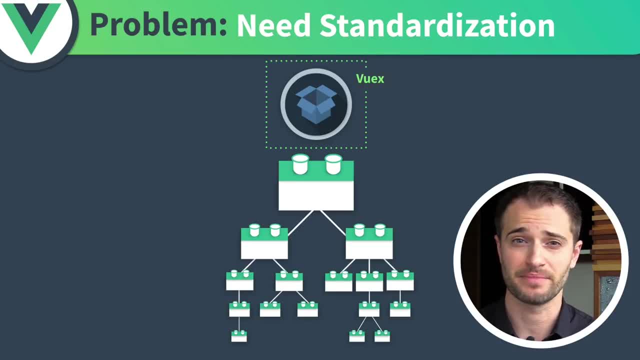 single source of truth doesn't fully solve the problems of state management. What happens when many different components alter the state in different ways from different locations? We need some standardization. Otherwise, changes to state can be unpredictable and untraceable. 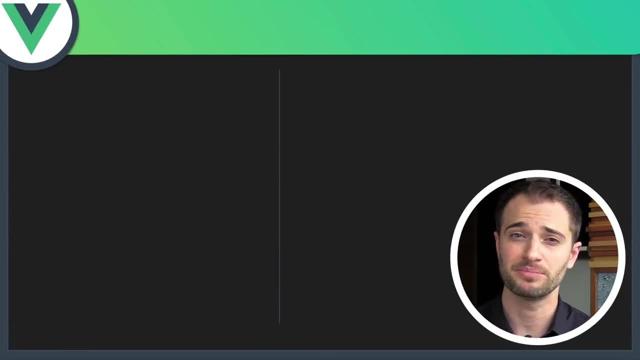 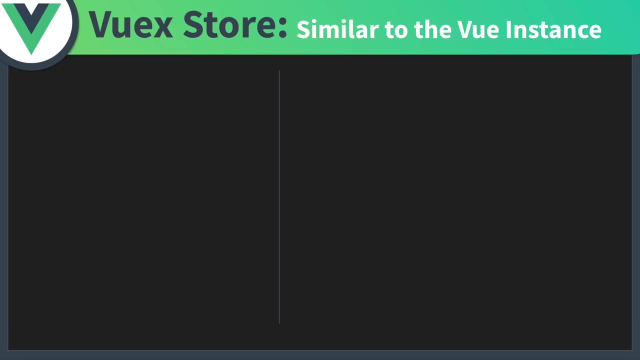 This is why Vuex provides a full state management pattern for a simple and standardized way to make state changes. And if you're familiar with Vue, Vuex should look pretty similar. Just like we create a new Vue instance, we can create a new VuexStore with new Vuex.Store. While the instance has data, the VuexStore has state, both of which are reactive. The Vue instance has methods, which, among other things, can update our data. While the VuexStore has actions, which can update the Vuex state. 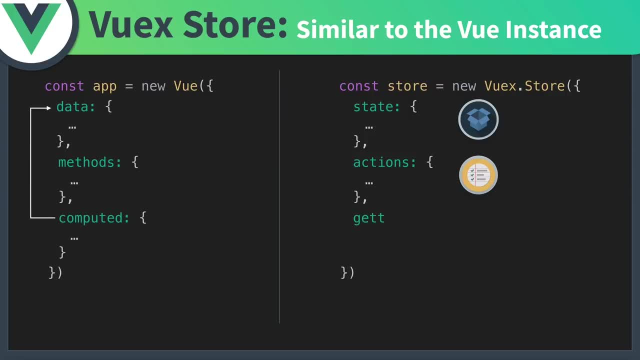 And while the instance has computer properties, which can access our data, the VuexStore has getters, which can access our state. The difference here is the store also, has mutations. Mutations are used to commit and track state changes. It's a best practice to have our actions call mutations, which update our state directly. And by using the Vue dev tools, we can do time travel debugging, and we can roll back a mutation, which reverts the state 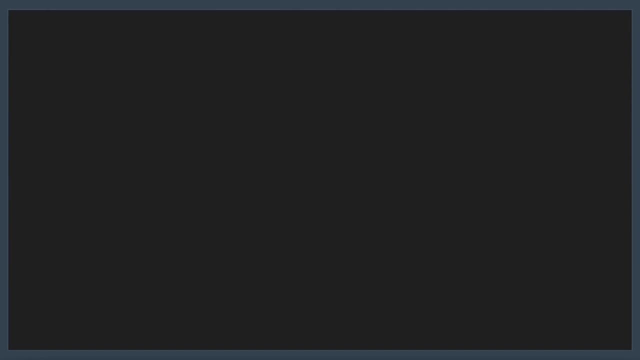 to its previous value. So let's look at an example VuexStore. In our state, we have a loading status, as well as a to-dos array. In our mutations, we have set loading status, which takes the state of our loading status and updates it. And we have set to-dos, which takes the state of our to-dos and sets it accordingly. Then in our actions, we have fetched to-dos. Let's walk through this code. 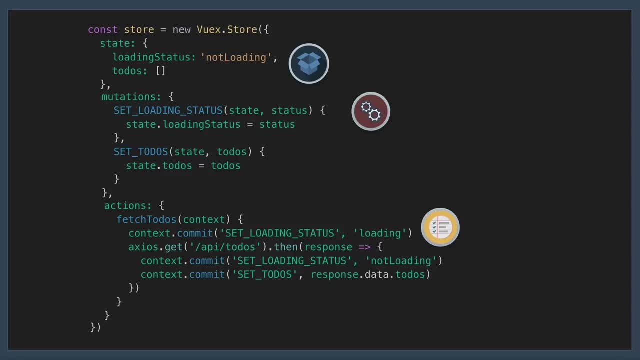 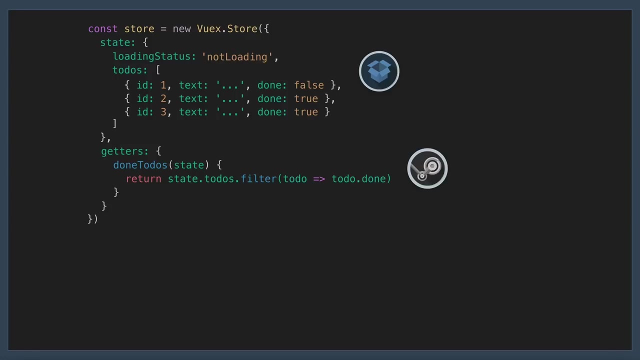 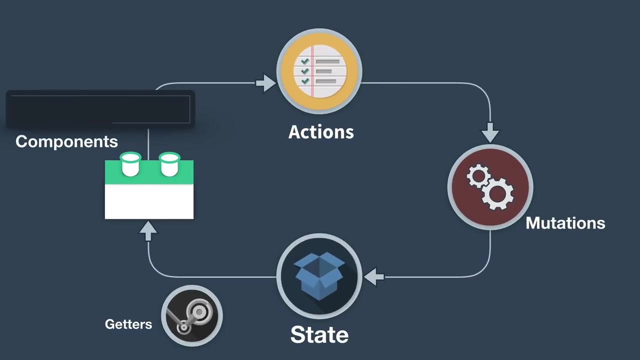 We're taking in the context object, which contains all the properties of our VuexStore, which allows us to commit mutations. The first mutation we're committing is set loading status, which will set the loading status to loading. Then we're making an API call. And when that response returns, we're going to set the loading status to loading. And when that response returns, we'll commit the set loading status mutation again, setting it to not loading. And finally, we'll commit set to-dos, setting the to-dos state with the response we got from our API call. If we need the ability to only retrieve the to-dos that are labeled done, we can use a getter for that, which will retrieve only the specific state that we want. Now let's look at Vuex in motion. From our component, we could dispatch the fetch to-dos action. And that'll be in the VuexStore VM. First, it'll commit the set loading status mutation, which updates our loading status state to loading. 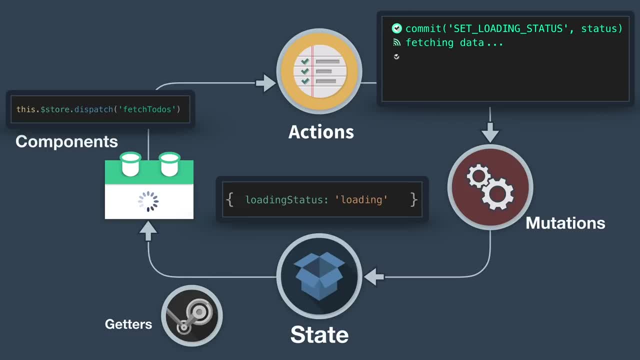 Then we'll fetch our data. And when that data is retrieved, we'll commit our set loading status again, updating our loading status. And here, we just need to load that data. So let's just make sure that the satisfactor is taken, and that's what we're going to do in this example. 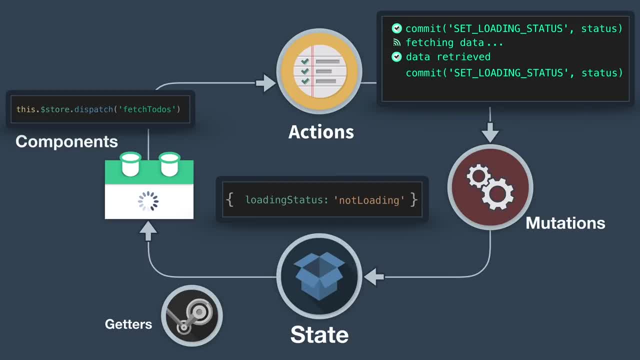 Now that we've created the set loading status mutation... We're going to remote our VuexStore VM is that, and then we're going to remote our VuexStore VM. We'll commit the token to that device, which is the very same yeah. So we're going to Bianca. We're going to enjoy the VuexStore VM, status to NotLoading. 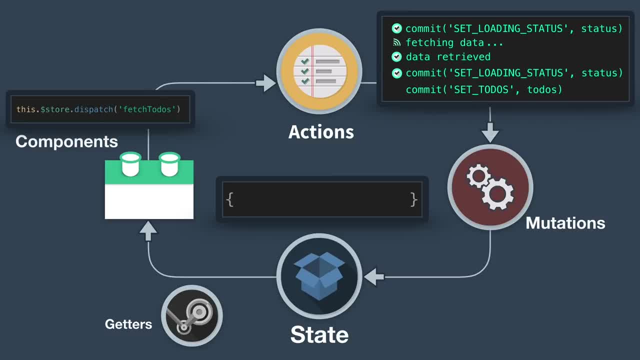 And finally, we'll commit the SetToDoes mutation, which sets the ToDo state with the API's response. And if we only wanted to get the DoneToDoes, we can use the getter to achieve that. 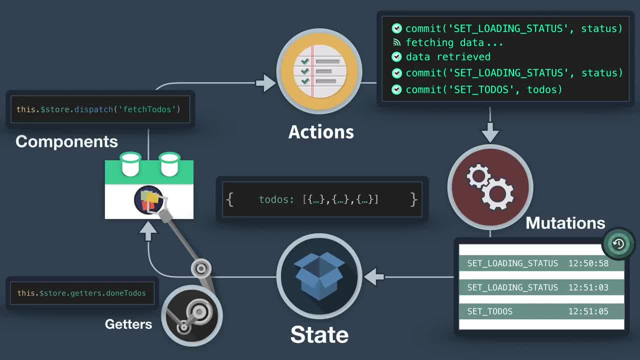 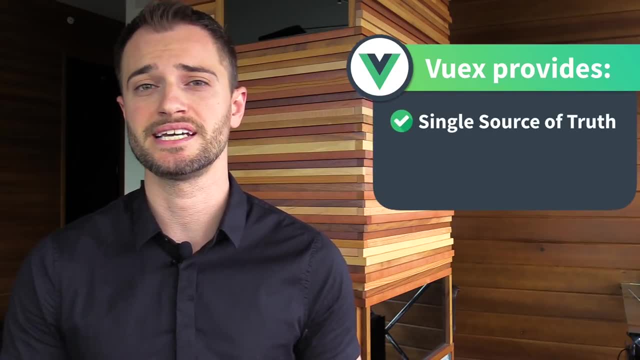 that was committed. Hopefully you now understand how Vuex can enhance your application by providing a single source of truth for your state and a useful library of actions, mutations, and getters. 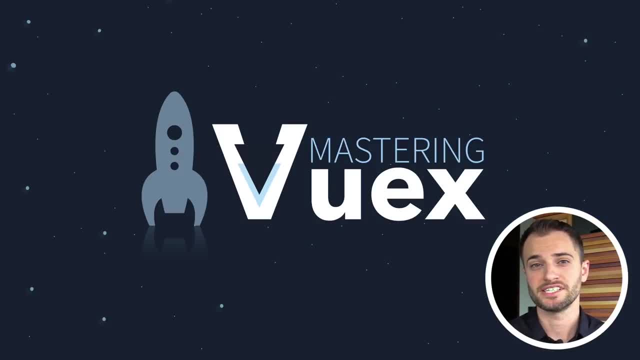 To continue learning about Vuex, you can check out the official Vuex documentation, or to continue learning with me, you can head over to VueMastery.com and watch our entire Mastering Vuex course. We have over an hour's worth of Vuex content. Hope to see you there. Thanks for watching.